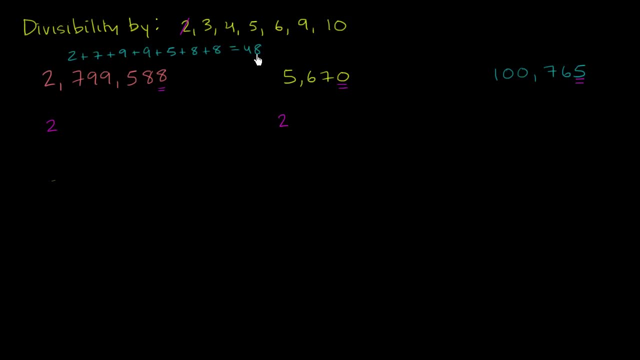 But in case you're not sure. so this is equal to 48.. In case you're not sure whether it's divisible by 3, you can just add these digits up again. So 4 plus 8 is equal to 12.. 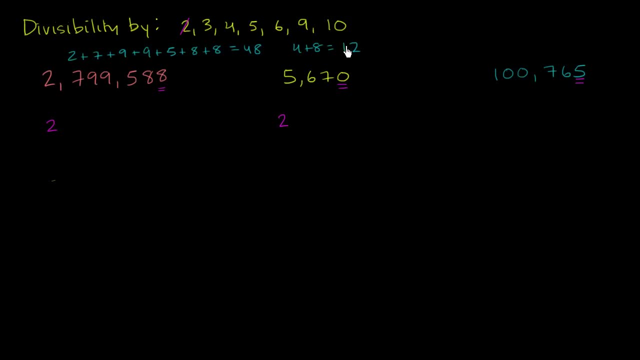 And 12 clearly is divisible by 3.. And if you're not even sure there, you could add those two digits up: 1 plus 2 is equal to 3. And so this is divisible by 3.. This right over here. 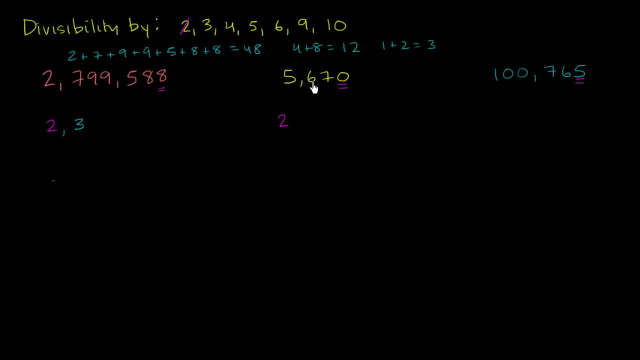 Add up the digits And we can do this one in our head pretty easily: 5 plus 6 is 11.. 11 plus 7 is 18.. 18 plus 0 is 18.. And if you want to add the 1 plus 8 on the 18,, you get 9.. 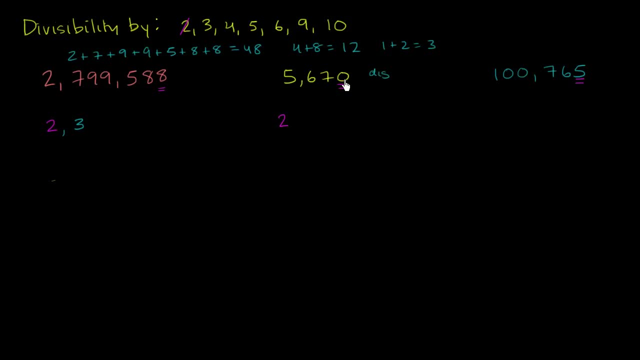 So the digits add up to 9.. Well, they add to 18,, which is clearly divisible by 3 and by 9.. And these two things will add to 9.. So the important thing to know is, when you add up all the digits, the sum is divisible by 3.. 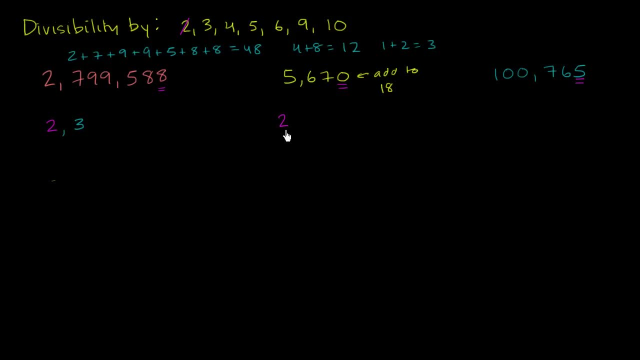 So this is divisible by 3 as well. And then finally, let's add up these digits: 1 plus 0 plus 0 plus 7 is 8.. Plus 6 is 14.. Plus 5 is 19.. So we summed up the digits. 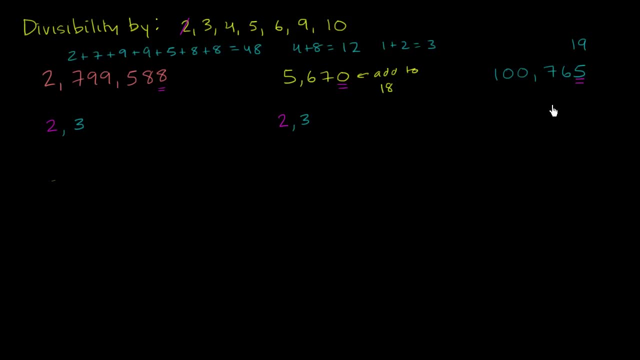 19- is not divisible by 3.. So this one- we're not going to write a 3 right over there- It's not divisible by 3.. Let's try 4.. And to think about 4, you just have to look at the last two digits and to see. 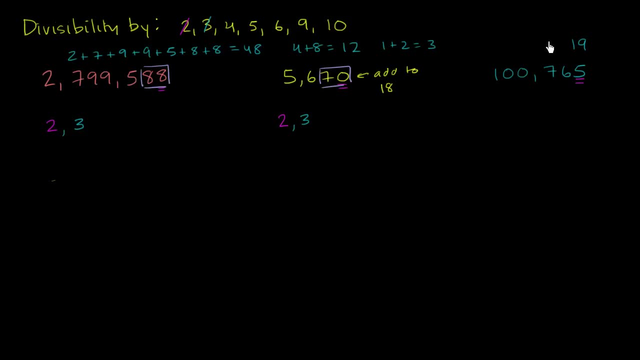 are the last two digits divisible? Are the last two digits divisible by 4?? Immediately, you can look at this one right over here. See, it's an odd number. If it's not going to be divisible by 2, it's definitely not going to be divisible by 4.. 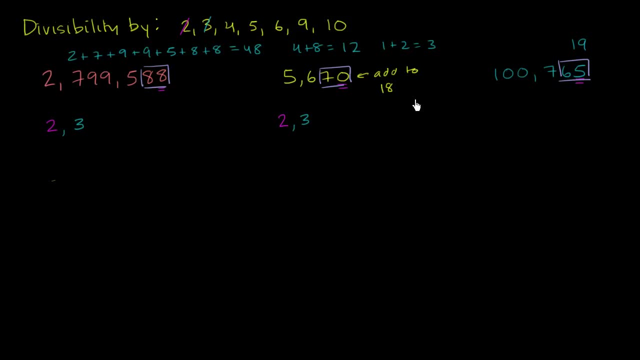 So this one's not divisible by any of these first few numbers right over here. But let's think about this one: 88, is that divisible by 4?? And you could do that in your head- That's 4 times 22.. 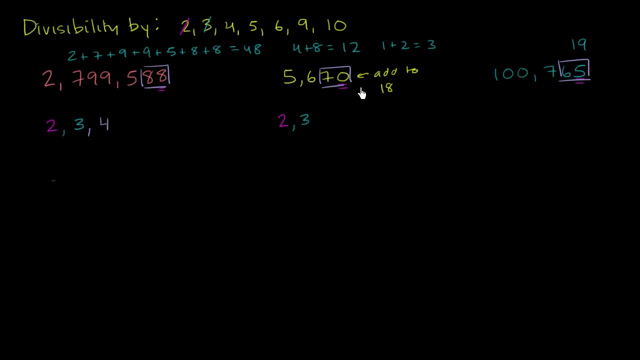 So this is divisible, Divisible by 4.. Now let's see: 4 goes into 60 15 times, And then to go from 60 to 70, you have to get another 10, which is not divisible by 4.. 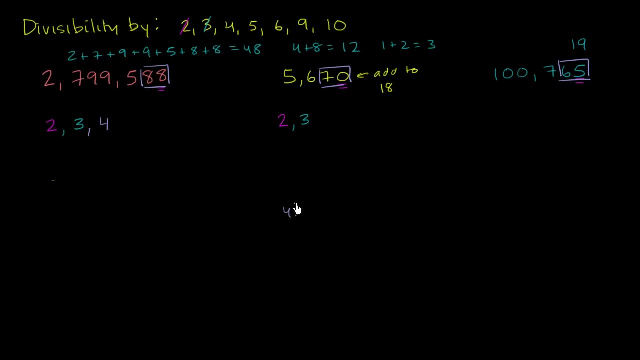 So that's not divisible by 4.. And you could even try to divide it out yourself: 4 goes into 70,. let's see: 1 times You subtract, you get a 30.. 4 goes into 30, 7 times. 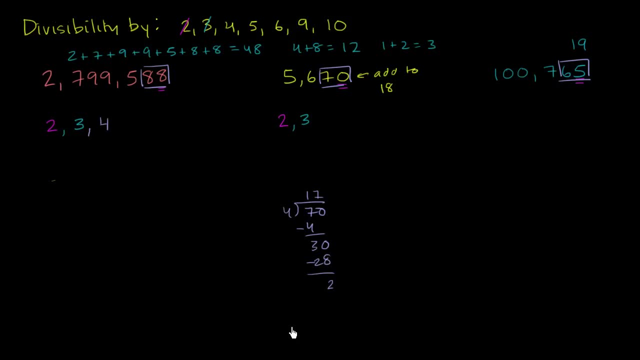 You multiply, then you subtract, You get a 2 right over here as your remainder. So it is not divisible, Divisible by 4.. Now let's move on to 5. And you're probably already very familiar with this. If your final digit is a 5 or a 0,, you are divisible by 5.. 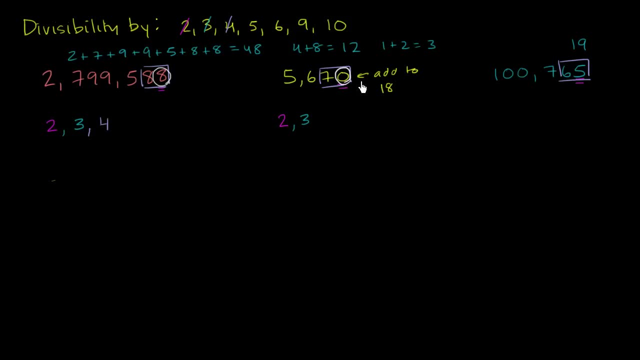 So this one is not divisible by 5.. This one is divisible by 5.. You have a 0 there, So this is divisible by 5.. And this you have a 5 as your ones digit. So once again, finally, this is divisible by something. 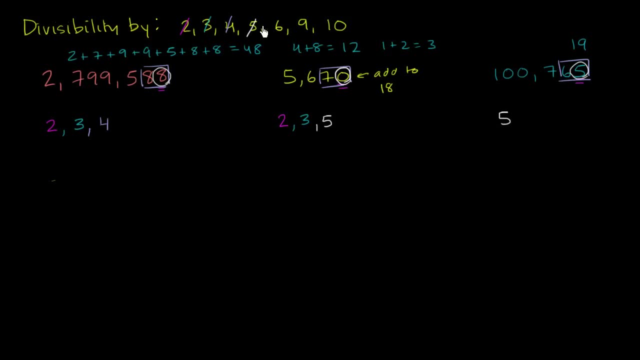 It's divisible by 5.. Now the number 6.. The simple way to think about divisibility by 6 is that you have to be divisible by both 2 and 3 in order to be divisible by 6. Because the prime factorization of 6 is 2 times 3.. 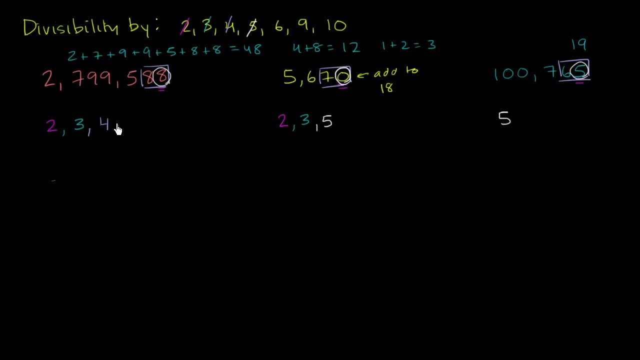 So here we're divisible by 2 and 3.. So we're going to be divisible by 6.. Here we're divisible by 2 and 3.. So we're going to be divisible by 6.. And if you were just divisible by 2 or 3, just one of them. 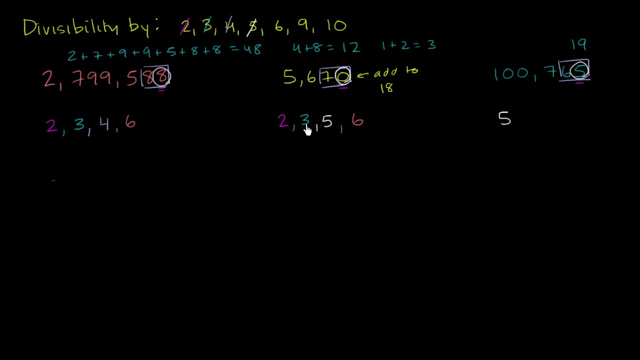 then you wouldn't be able to do this. You have to have both a 2 and a 3. Divisibility by both of them. And here you're divisible by neither 2 nor 3. So you're not going to be divisible by 6.. 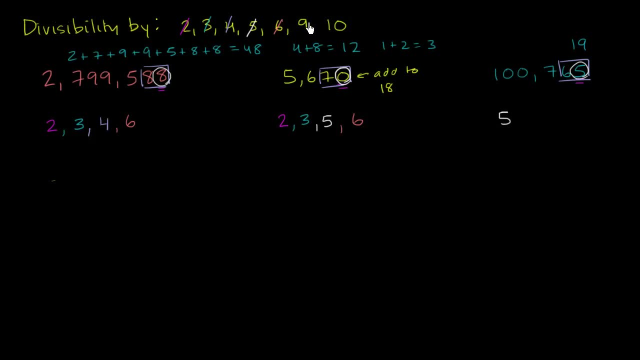 Now let's do the test for 9.. The test for 9 is very similar to the test for 3.. Sum up all the digits. If that sum is divisible by 9, then you're there. Well, we already summed up the digits here. 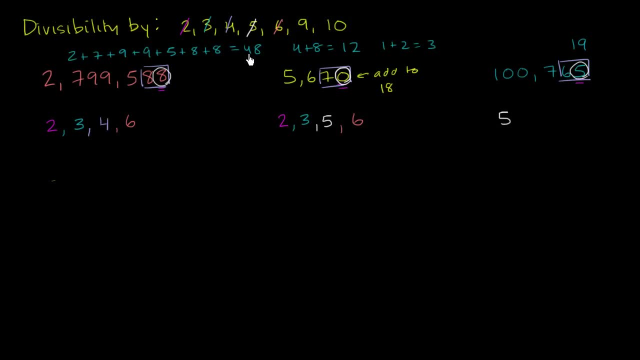 48 actually is not divisible by 9.. If you're not sure, you can add up the digits. there You get 12.. 12 is definitely not divisible by 9.. So this thing right over here is not divisible by 9.. 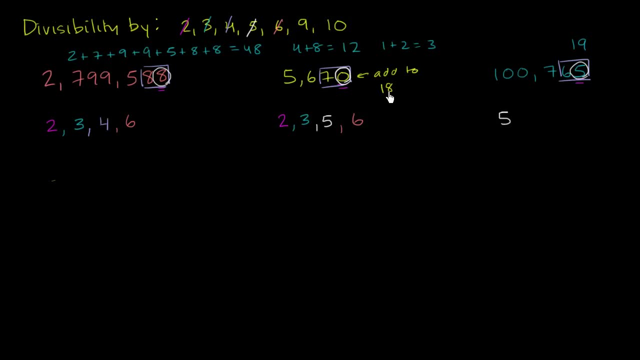 And this one over here. if you added up all the digits, we got 18, which is divisible. It is divisible by 9. And I'm running out of colors, So this one is divisible by 9. All the digits added up to 18.. 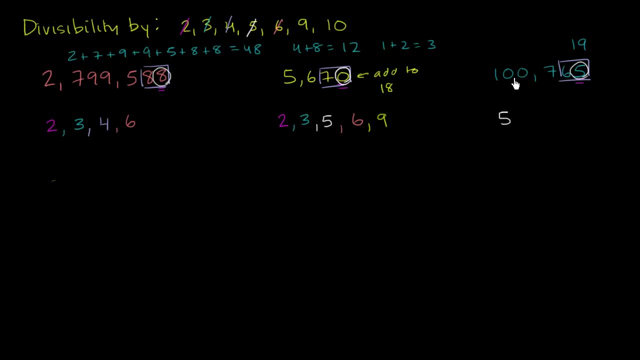 And this one over here. you don't even have to add them up, Because we already know it's not divisible by 3.. If it's not divisible by 3, it can't be divisible by 8.. But if you did add up the digits,